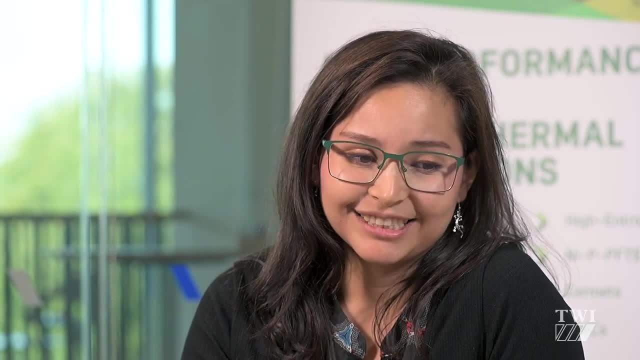 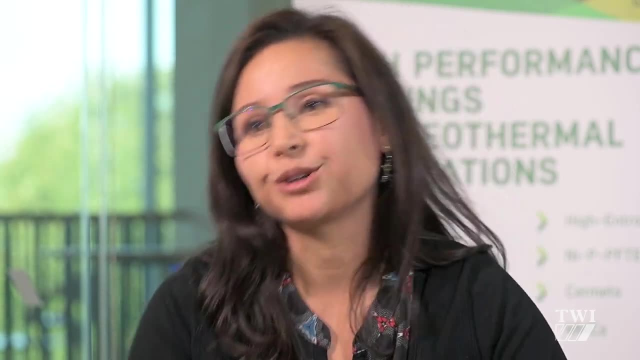 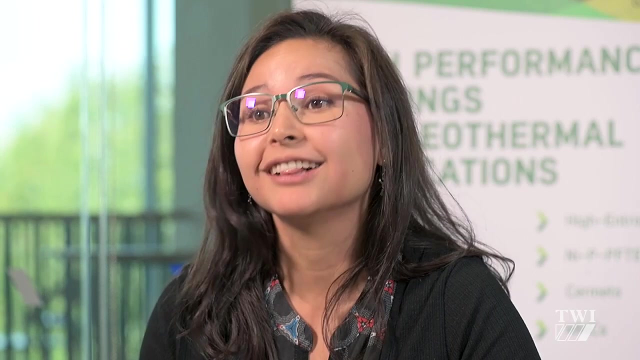 So I work in the field of rock mechanics and what we know is that there is very little knowledge on how pressure and temperature and geochemistry is in the subsurface, because it's really hard to reach five kilometres depth until we have drilled a well. So what we do with rock mechanics? 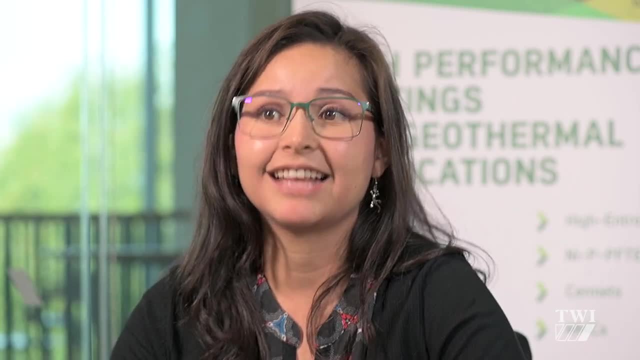 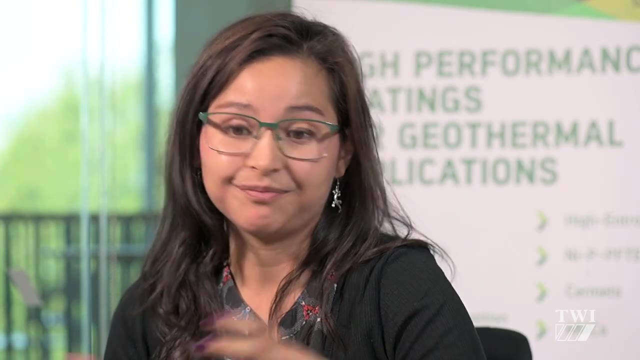 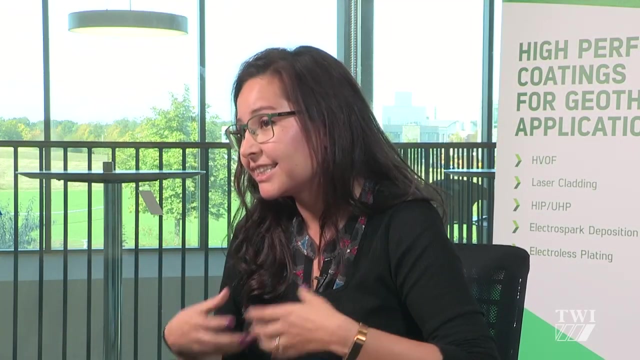 is to try and theorise and then experiment into what are the influences that this differential pressure has in, like the aperture of fractures, and that has a big impact on how permeability evolves in the, in the reservoir, so like how fluids are going to be flowing towards the surface and how effective our 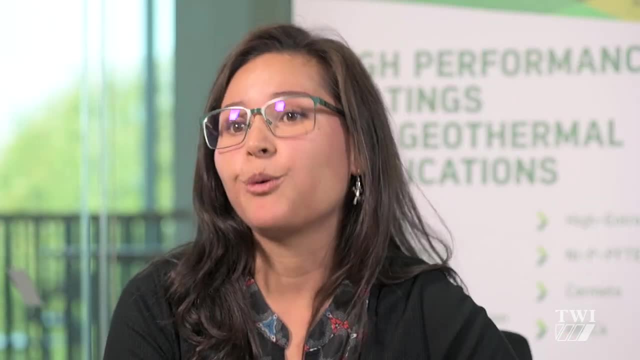 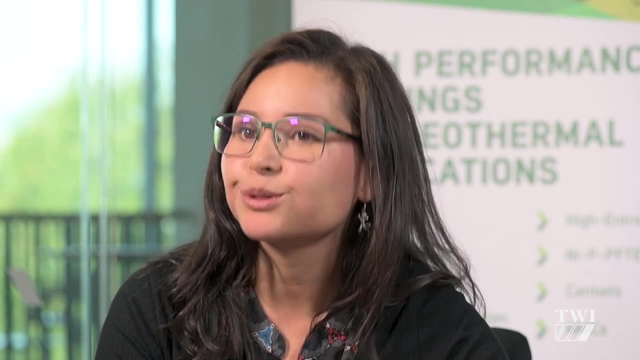 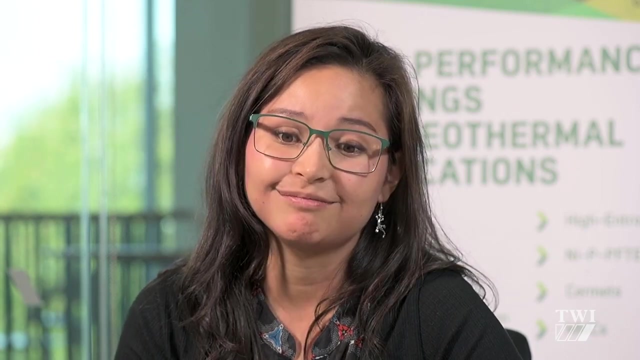 reservoir is going to be is highly dependent on knowing the permeability. So rock mechanics is a tool that we use and we go to the lab and we do some experiments to try and figure out what can be the conditions underground. So I think they're both really important techniques, both rock mechanics and 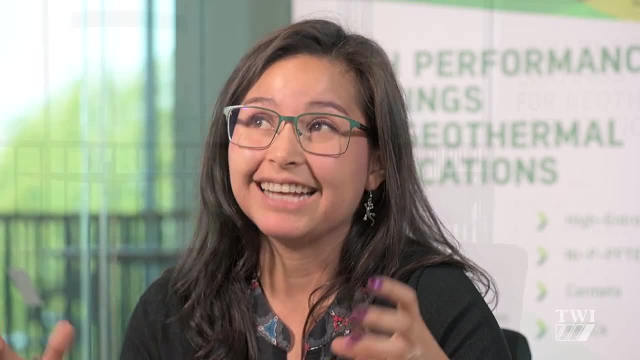 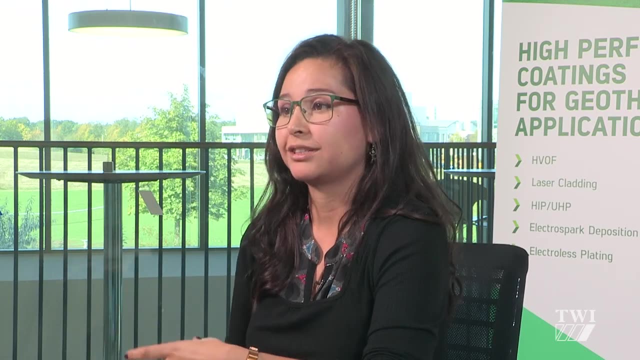 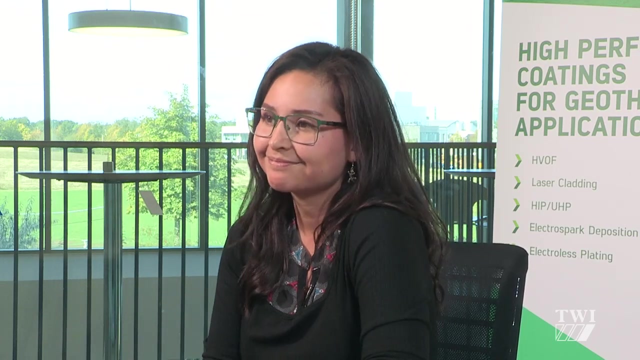 geochemistry, because the geochemical part- it's also very important to know the conditions underground. Minerals transform and they change the physical properties of the rock. so when you put those two techniques together you can have a much better idea of the subsurface. Well, I think in Science for Clean Energy we have a very unique 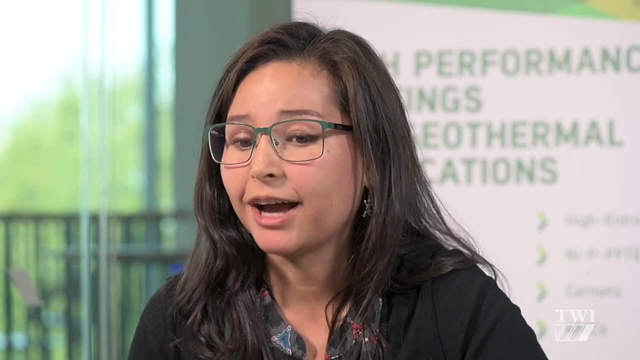 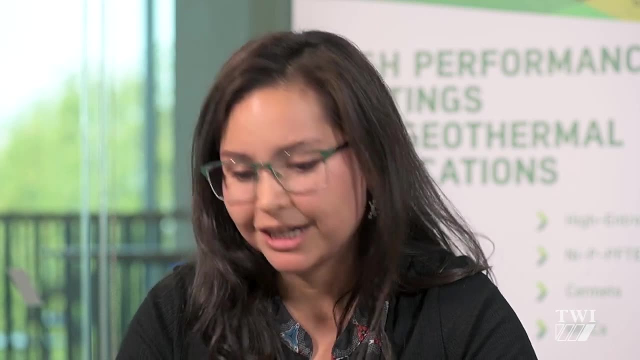 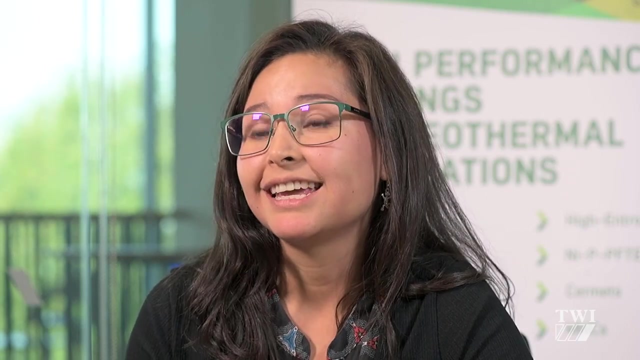 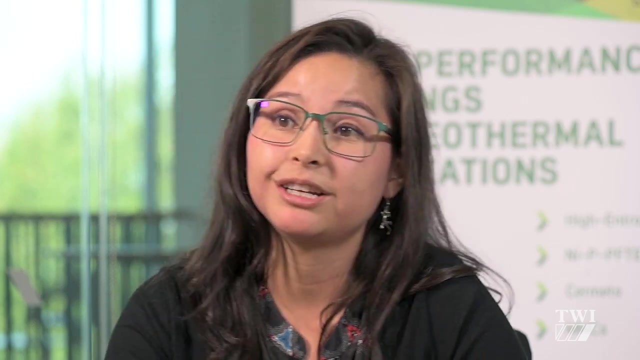 opportunity, because the project combines 32 partners that come both from academia and from industry and they share really different sorts of expertise and in this way, what the aim of the project is is to assess the risk of exploiting the subsurface in general. So having a partners that are actually really 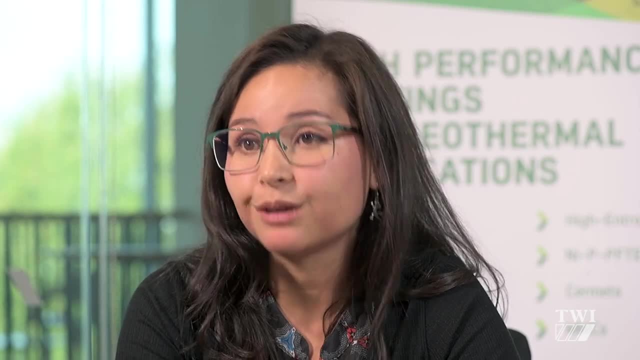 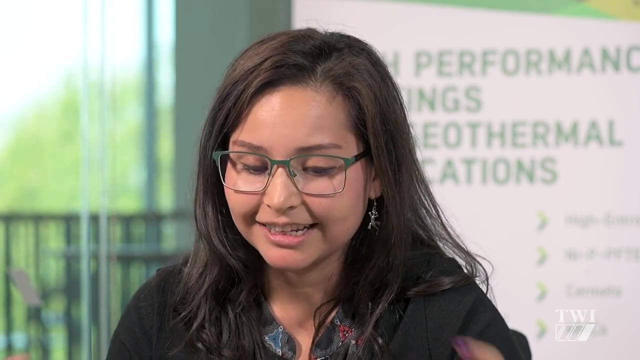 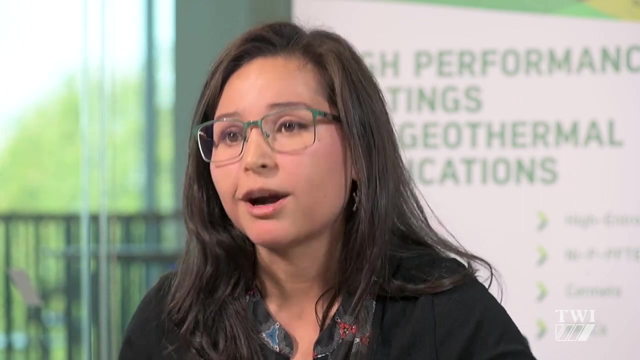 operating the wells, like the United Downs geothermal system, and on energy in Iceland. they allow us to have access to the wells, to have access to the reservoirs, to know the areas, and all these partners can like really learn from that, deploy their new technologies and assess the 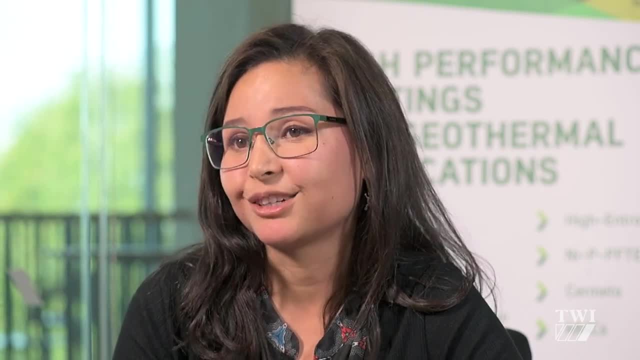 risks and find ways to improve it in general. So I think the project is definitely doing great.